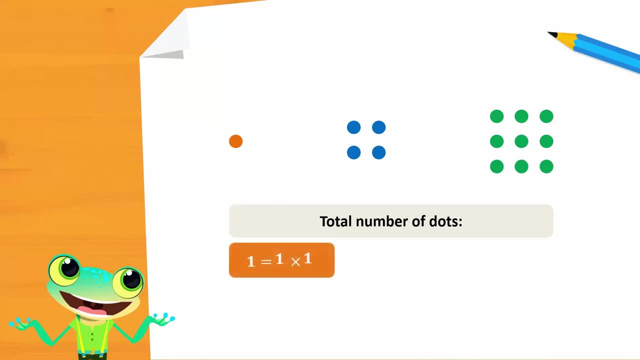 columns is also 1.. So we have 1 times 1, which is equal to 1 dot. In the second group, there are 2 rows and 2 columns, So we have 2 times 2, which gives us 4 dots. In the third group, there are 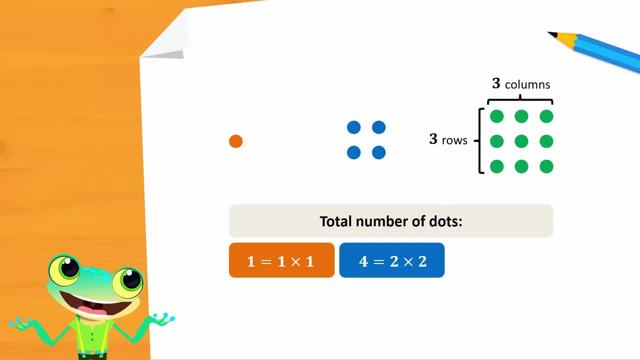 3 rows and 3 columns, So we have 3 times 3, which gives us 9 dots. Do you notice any patterns in these three statements? Each number- 1,, 4 and 9- is the product of a number that is multiplied by itself. 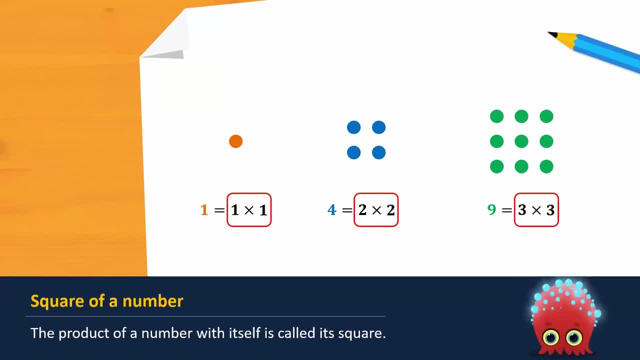 The product of a number multiplied with itself is called its square. So 1 is the square of 1, 4 is the square of 2 and 9 is the square of 3.. A square is denoted by writing a small 2 at the top right of a number. 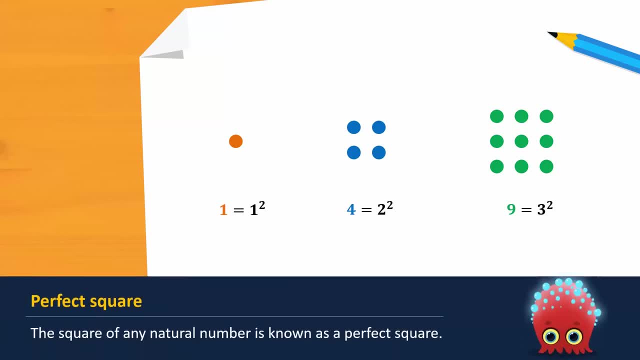 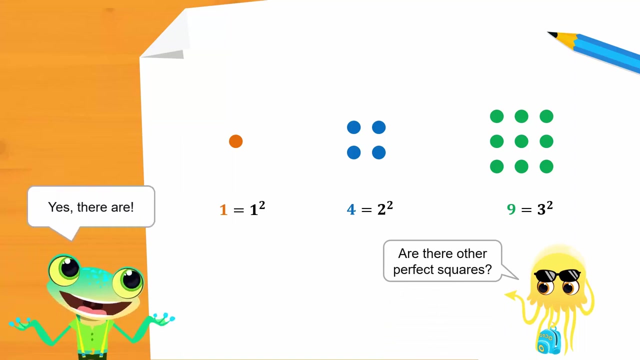 The square of any natural number is known as a perfect square. Since 1,, 2 and 3 are natural numbers, their respective squares 1,, 4 and 9 are all perfect squares. Are there other perfect squares? Yes, there are. We can form more perfect squares by finding the square of other natural numbers. 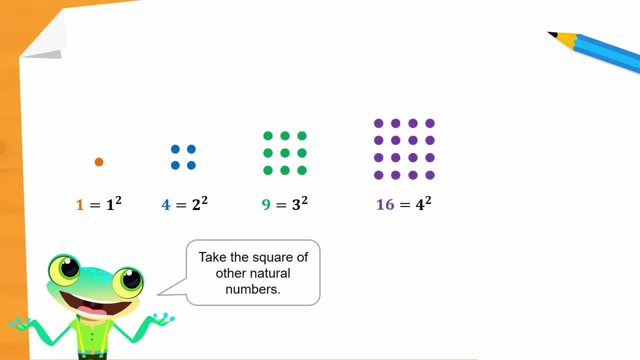 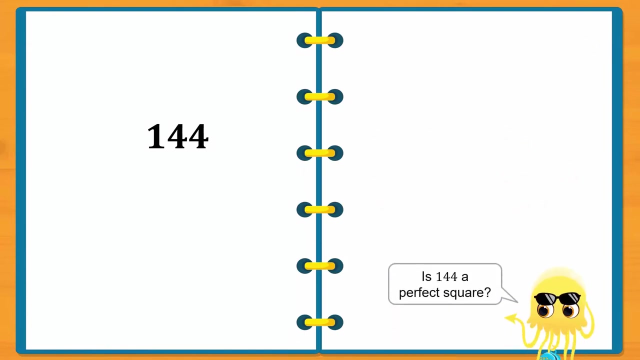 For example, 4 squared is 16,, while 5 squared is 25.. So both 16 and 25 are perfect squares. Now, given a number such as 144, how do we check if it is a perfect square? We don't want to draw 144 dots and try to arrange them into a square shape. 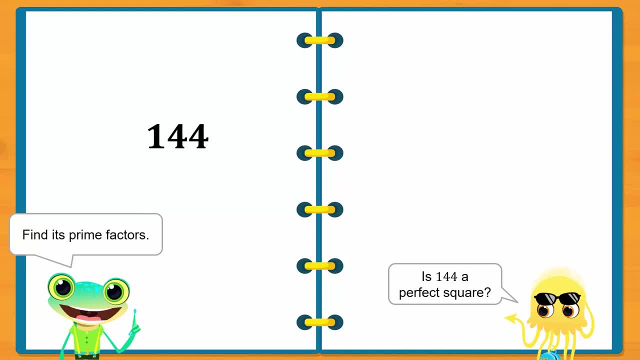 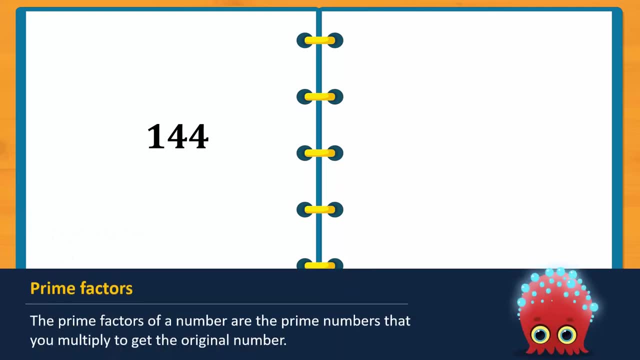 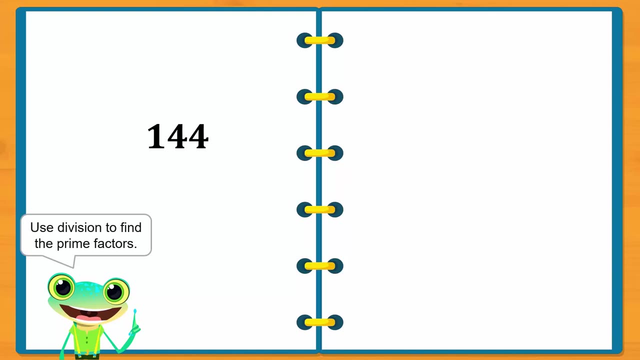 We do so by first writing the number as a product of its prime factors. The prime factors of a number are the prime numbers that you multiply to get back to the original number. We use division to find prime factors. We use division to find prime factors. 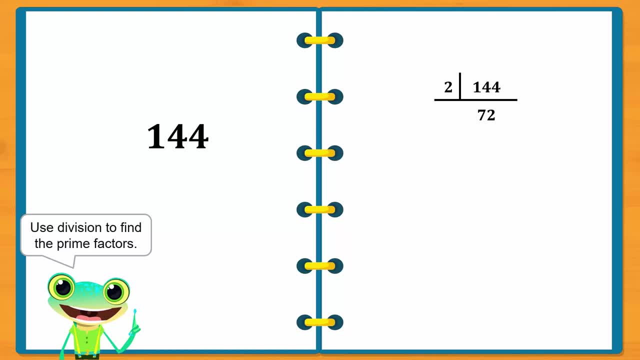 First divide 144 by its smallest prime factor, which is 2.. This leaves us with 72.. Next we divide 72 with its smallest prime factor, which is also 2.. We repeat this process until no further division can be done. 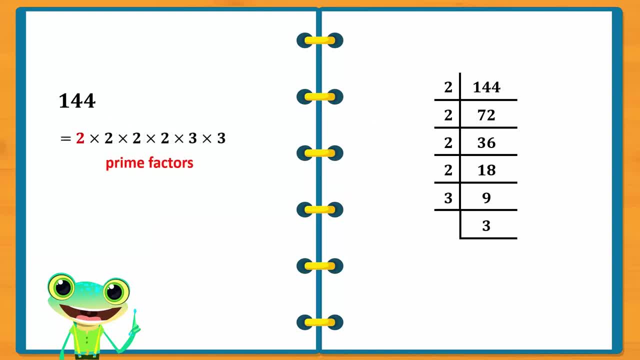 The prime factors of 144 are therefore 2, 2, 2,, 2,, 3, and 3.. Next group similar factors into pairs. 4 copies of 2 can be grouped into 2 pairs of 2.. Both copies of 3 are simply grouped into a pair. 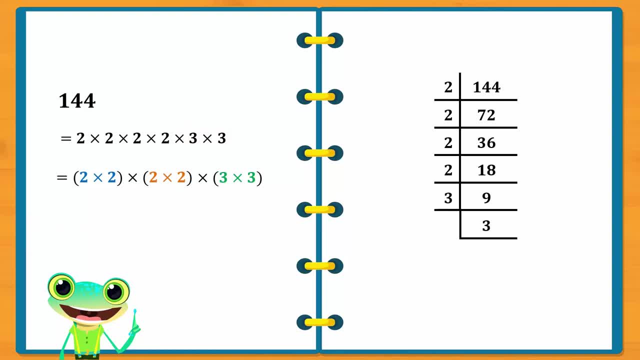 Therefore, every factor is part of a pair. When this happens, we can conclude that the number is a perfect square. Let's try another number: 16,875.. Again, we find its prime factors. The prime factors of this number are 3, 3,, 3,, 5,, 5,, 5, and 5.. 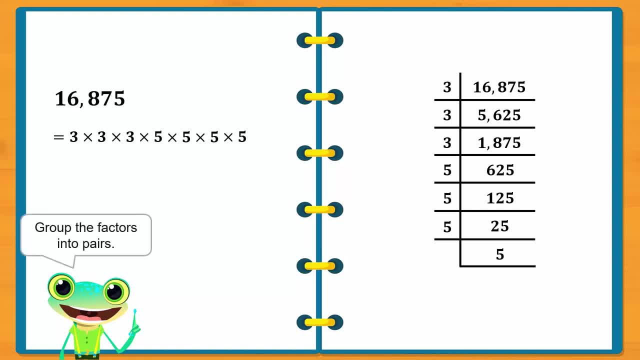 Next, group similar factors into pairs. Since there are 3 copies of 3, we will group them into pairs. You only have one pair of 3.. 4 copies of 5 can be grouped into 2 pairs. Here we see that this 3 is not part of a pair. 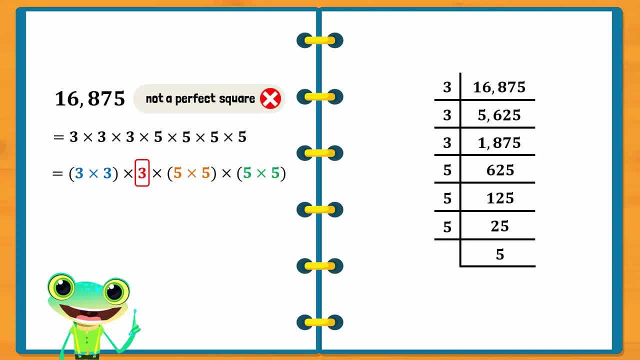 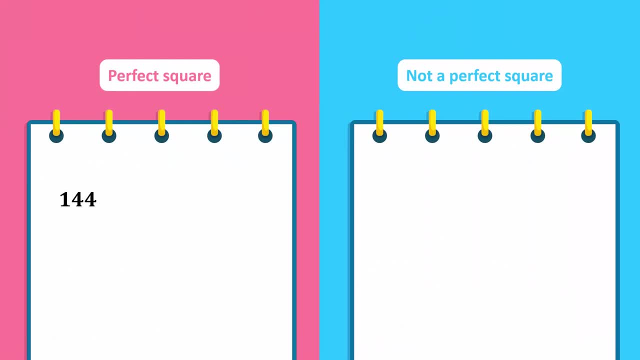 When this happens, we conclude that the number is not a perfect square. Therefore, to see if a number is a perfect square, first we list down all its prime factors and then determine if all the factors can be paired up. If not, it is not a perfect square. 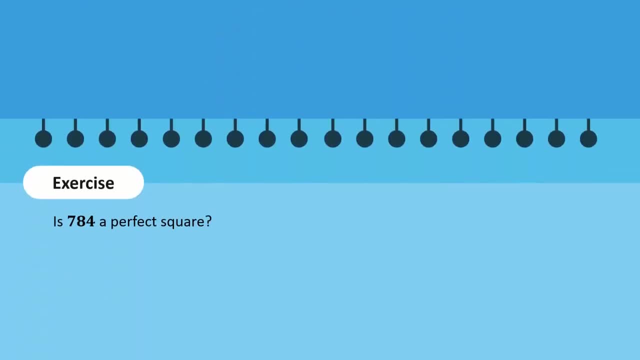 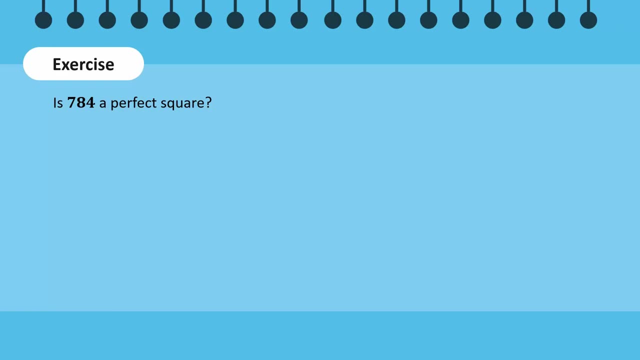